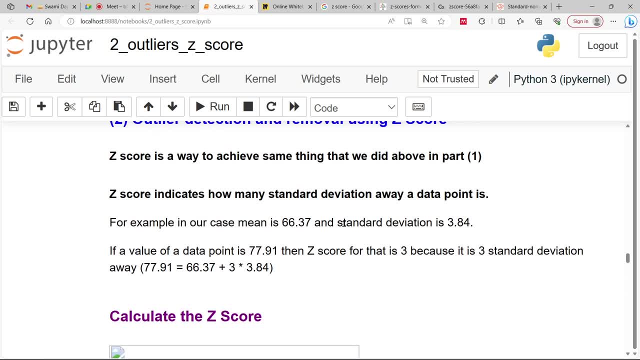 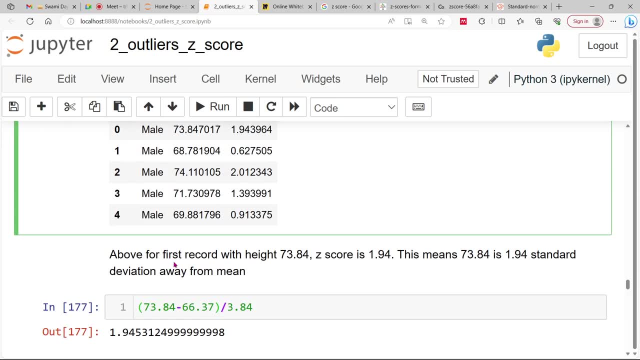 right, we have this that is called formula. for example, our case standard deviation is this one. we have just that formula for this one. so above four, first record, the height of 70 wave for a 3.84 z square is this one. this means 73.81 standard deviation away from me. 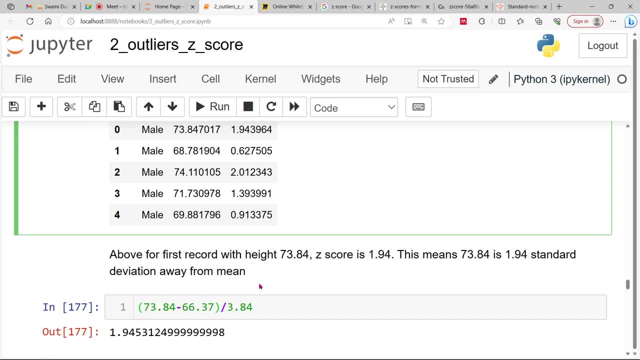 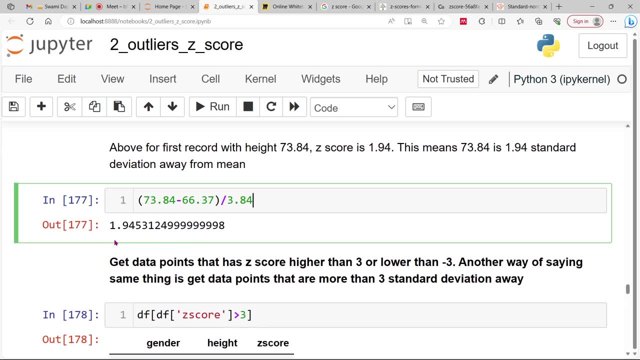 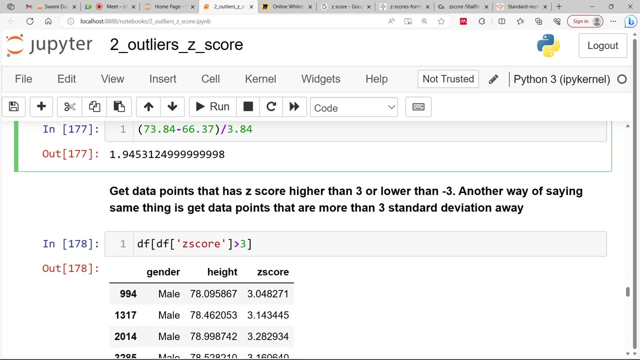 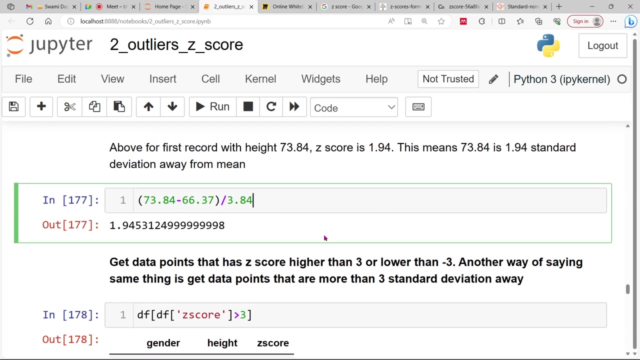 right, it's a 1.94 standard deviation away from me. right, then we have get points z square, then three and minus three. so you see, kabi, when we have greater than or equal to three, so we are going to discard these values, which is having three standard deviation. right, so we have three. so in 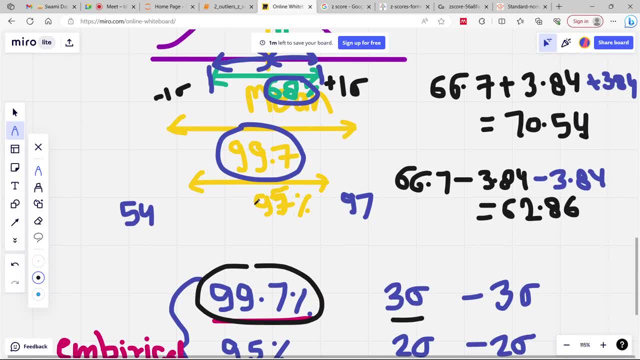 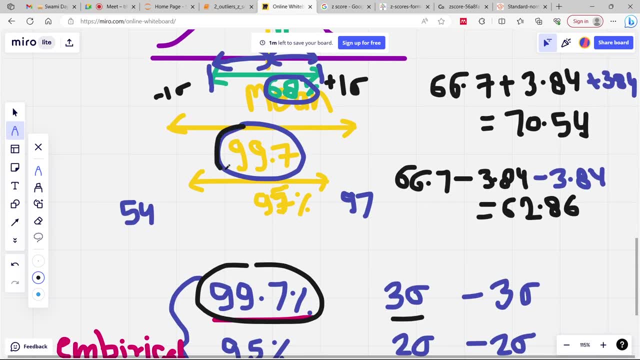 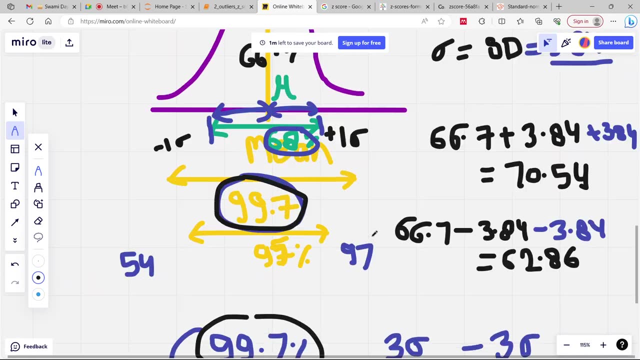 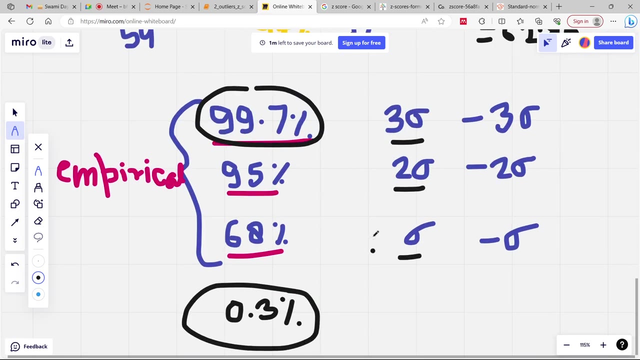 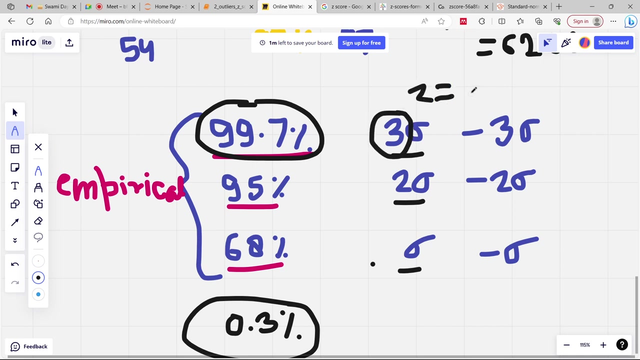 this formula where we have calculated this, values this, where we had 99.7 and all. so what is the maximum score? we selected this 99.7, so 99.7. what you did on both sides, you removed it. so once you have chosen this formula means you have selected z as a 3, right as a 3 you had 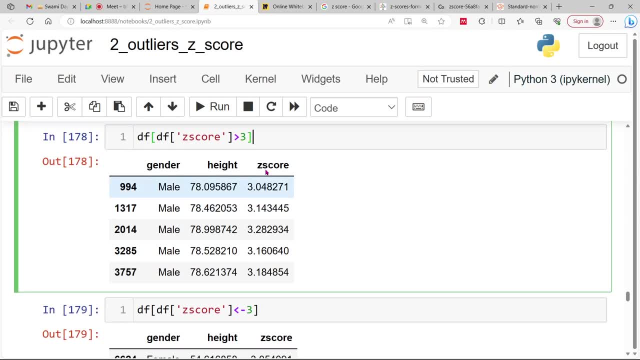 selected on the both side. now, if you are selecting this- 3 means beyond 3- you are selecting, you are discarding these values. so here we have 9, 1, 2, 3, 4, 5. these 5 elements are we are going to remove. 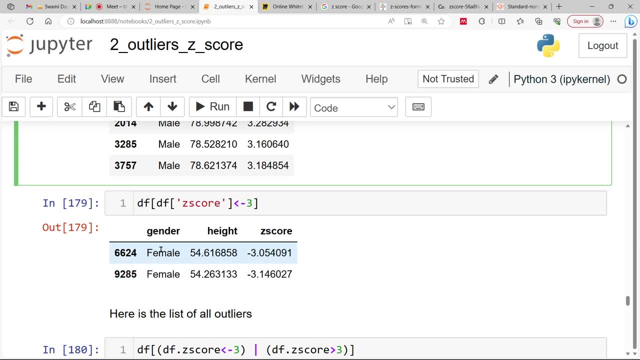 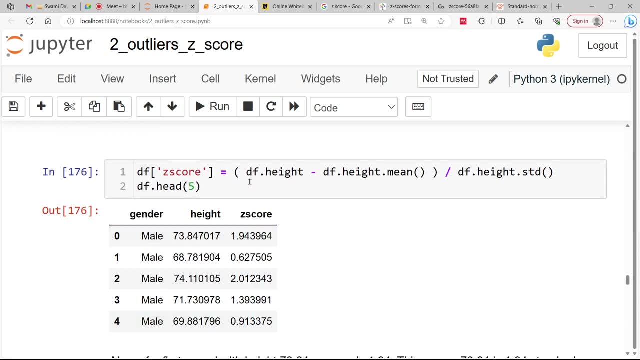 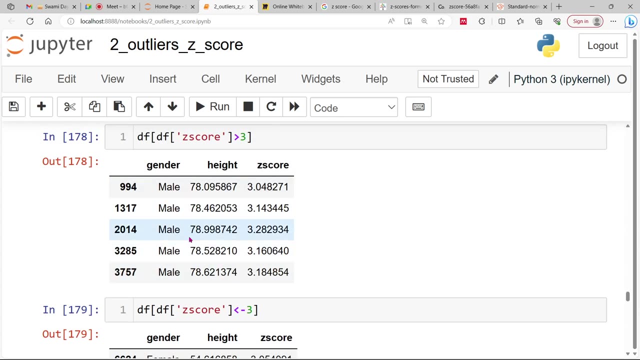 and when we have z less than minus 3, these two elements, candidates, are having less than 3 elements, z score, which we have calculated from the next column here using this formula. so now, beyond the range of these two, these 5, these 6 elements like 5, 6, 7, 7, and candidates those 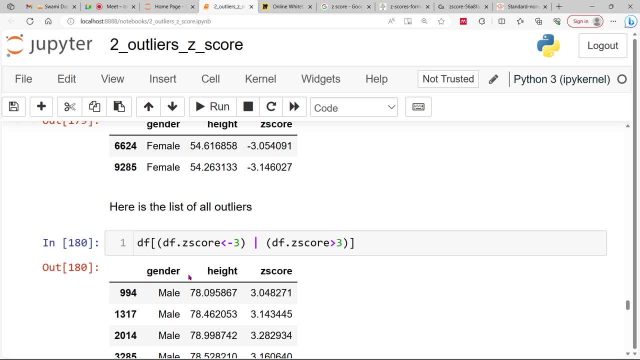 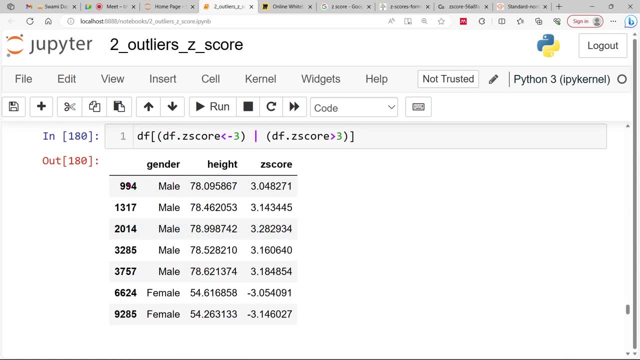 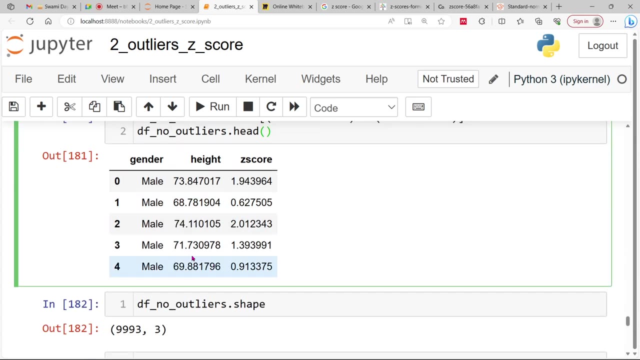 are not falling in this category, or you can say 3 z score or minus 3 z score. beyond these 7 candidates are coming. so I am going to collect these values, all these candidates, and finally remove the outliers and produce new data from. so this is the clean data set which has removed z score on the both side: 3 or minus 3k. 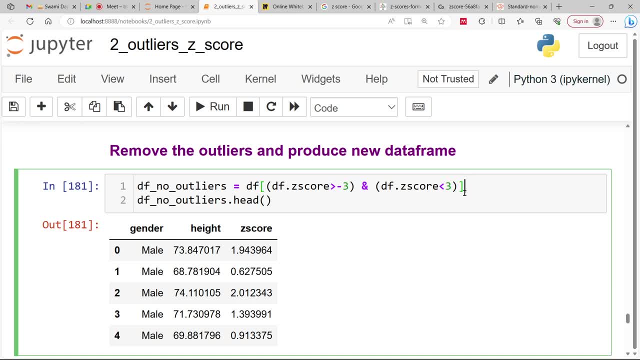 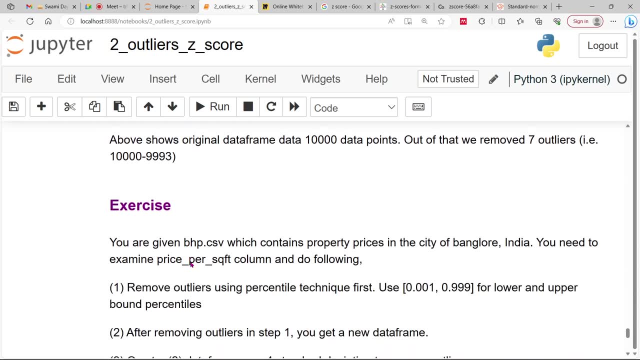 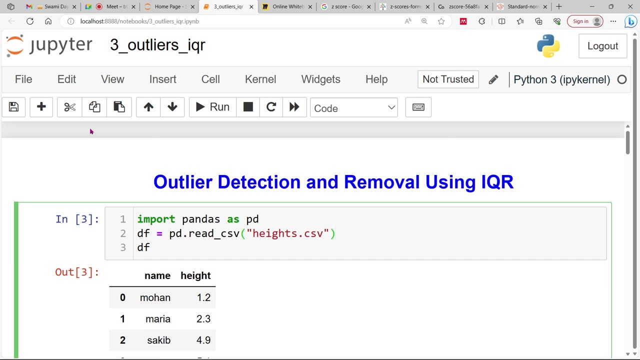 beyond. go remove Carnegie. can you pick up the main idea? now you have removed the outlets or you have the clean data set and then you can go ahead. do we have any query? okay, so in the third formula we are going to remove the outlet using IQR formula and we will see what is it. first, let me 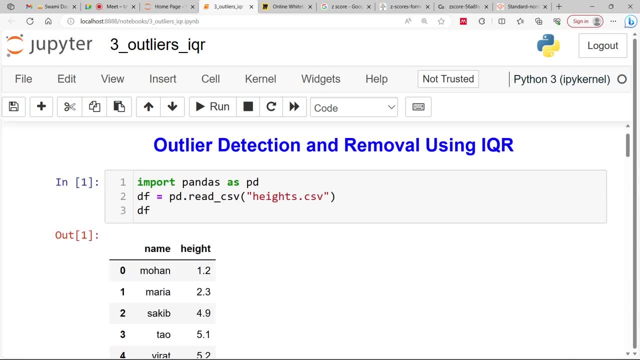 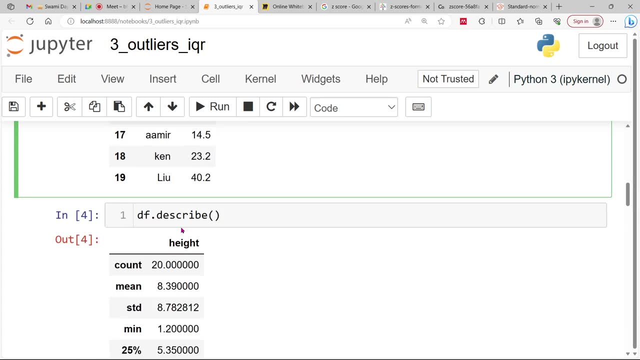 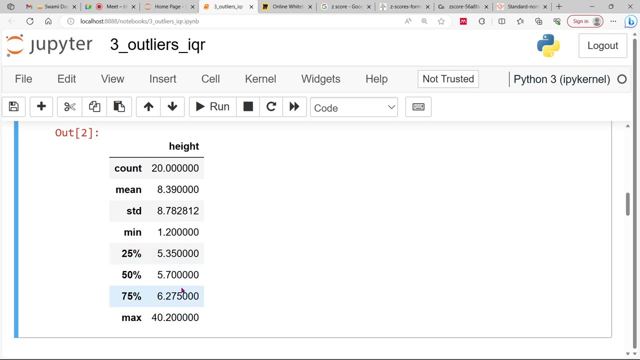 describe the data set. what kind of data set we are taking away? we are taking this data set where we have heights, right name and heights will be there. and then we have described the formula here you can see: standard deviation is 8 right, minimum is 1.2 percent. this one- and detecting outlets using this. 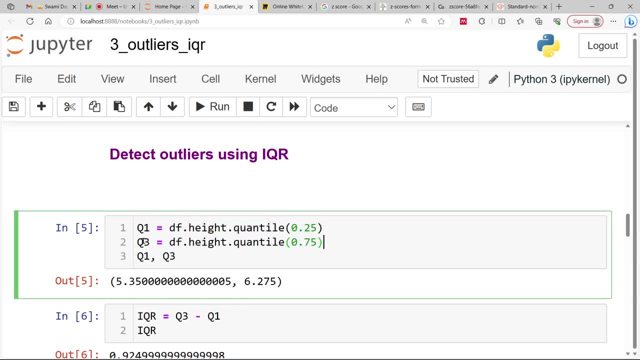 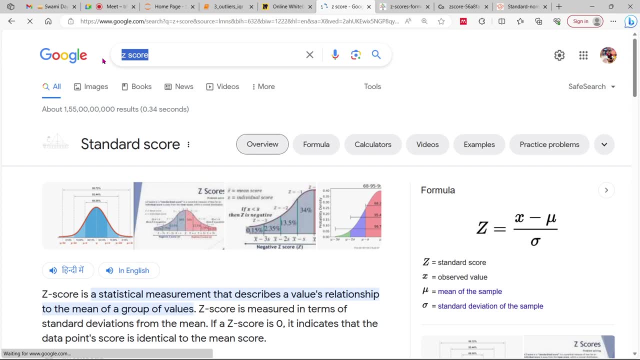 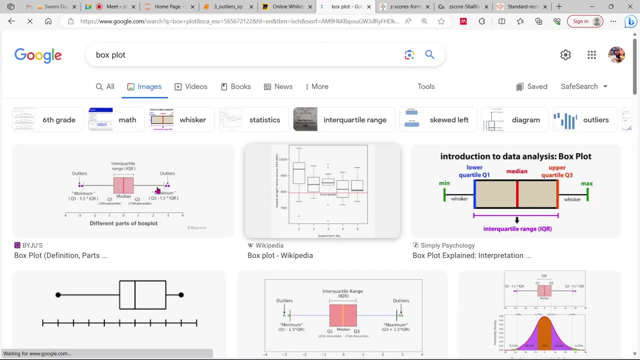 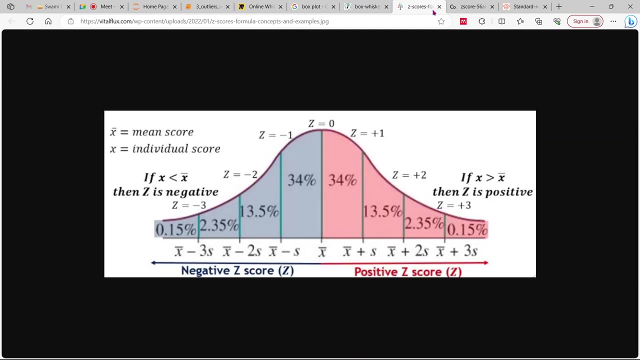 one first, what we have find out. we have find out 25 percent, 75 percent. okay, let me go ahead here. we have box plot. let me show you box plot value. so this image showing box block- certain properties are there associated within the given- is here we have lower quartile right. 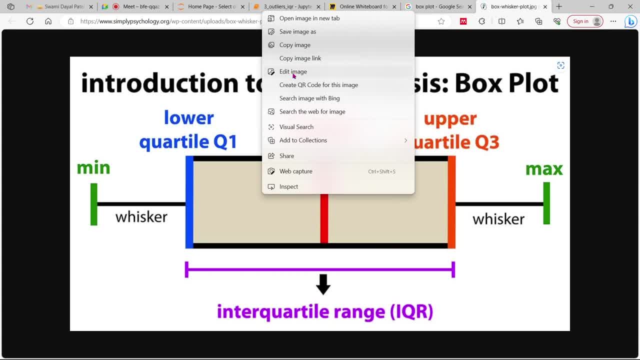 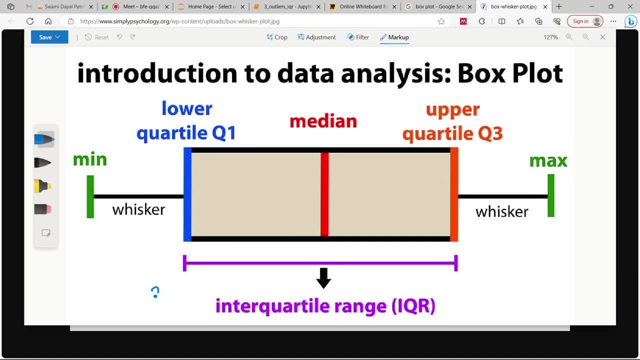 what is the lower quartile? in this lower quartile we have? this is called 25 percentile somewhere right, and here we call it 75 percent, right? this is the median means. this is 50 percentile, right? so this is percentile. we had discussed yesterday session. percentile is different from percentage, so we are having 25 percentile and 50. 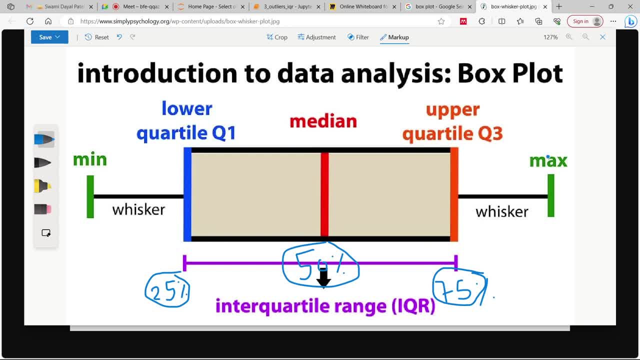 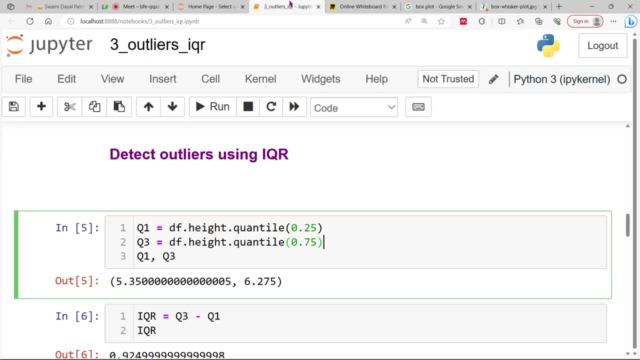 percentile. beyond above, we have mixed 75 percentile. what is this maximum and what is this minimum value? it's not the minimum value out of the given data set, or in other words, it's not the maximum value of above all the data set. it's something else. what? 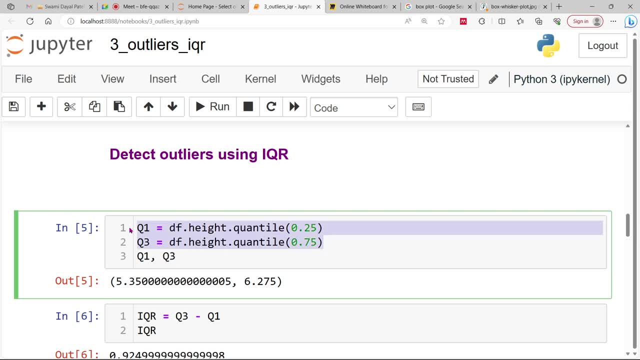 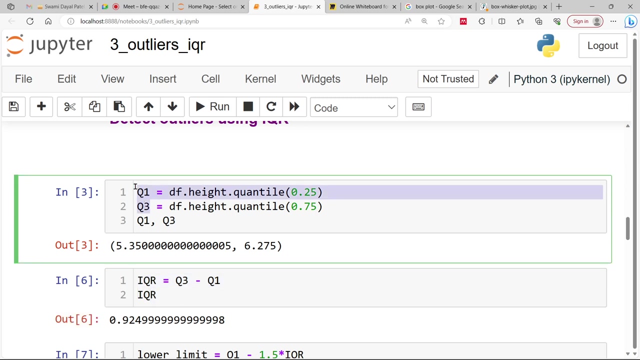 it is I'm going to explain. so let me explain this: q1 and q3. this is q1, first quartile. this is 25 percentile. q3 is worth 75 percentile. so I have taken quantiles, percentage, and then 0.25, which is giving around 5.35 and 6.75 respective. now I'm giving IQR. IQ is what q3. 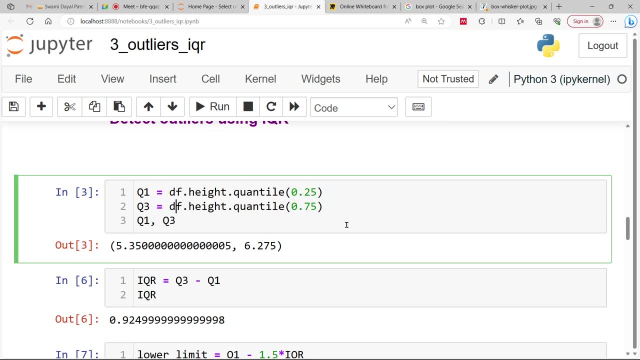 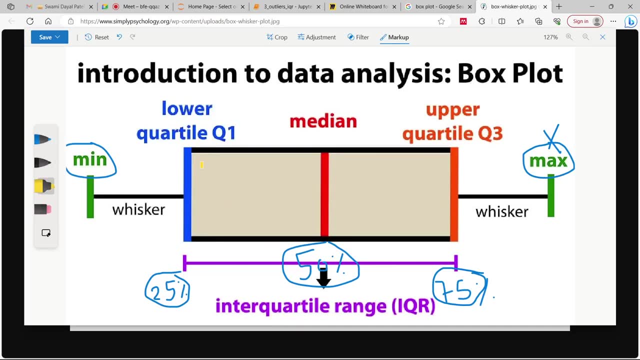 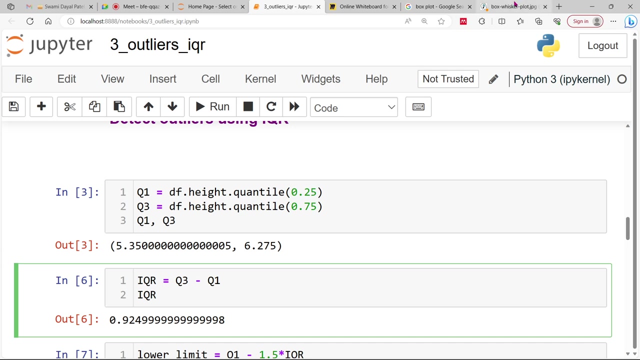 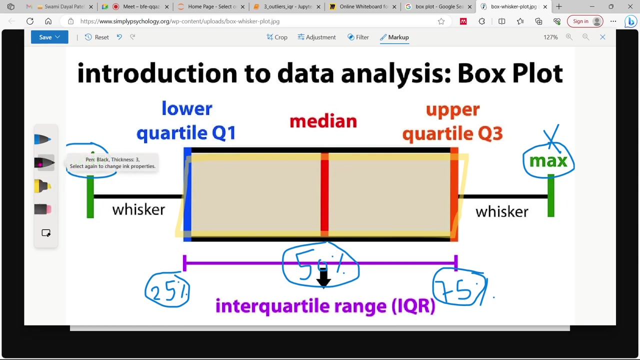 minus q1, which is giving difference between 75 percentile and 25 percentile. go back to my box plot here you can see this box is kind of. this box is kind of: I, E, Q, R, right, inter quant quantile range, right, you can see this is so having. 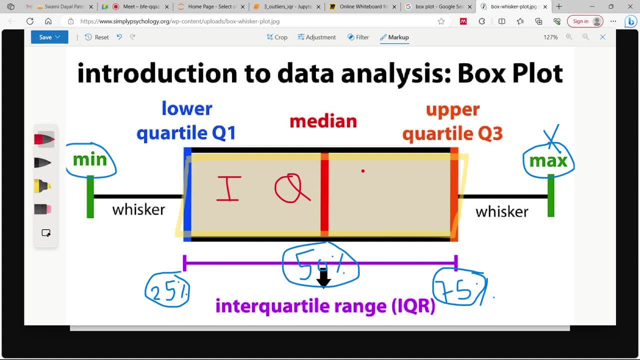 this is I E Q R box, where we have this values, and here we have lower quartile and the upper quartile right. once I will get the difference between Q 3 minus Q 1, I'll get the range of this IQR interquantile range. so this is what IQR. 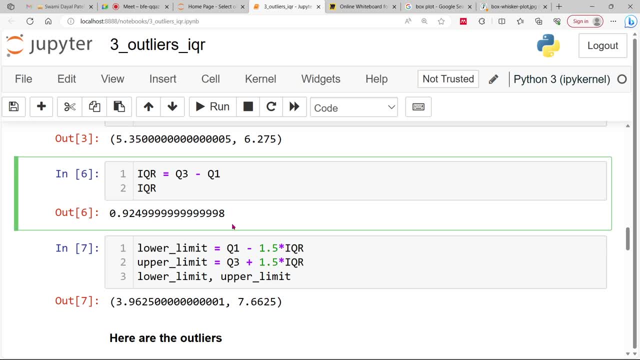 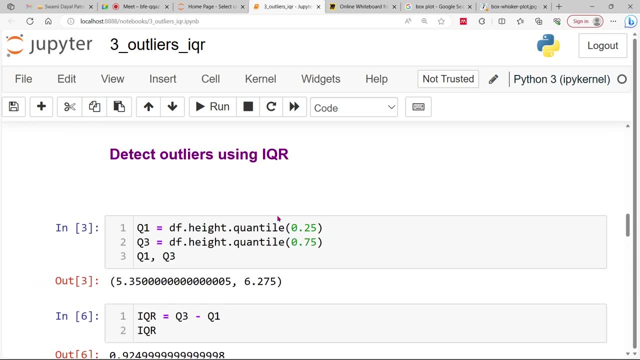 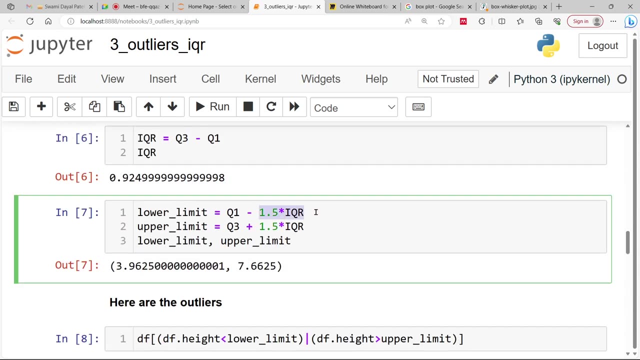 q 3 minus q 1.. we can see this is 4.925, something now lower limit. so lower limit is what q1 minus q 1 is? what if twenty five percentile, when you subtract twenty five percentile minus 1.5 of IQR? 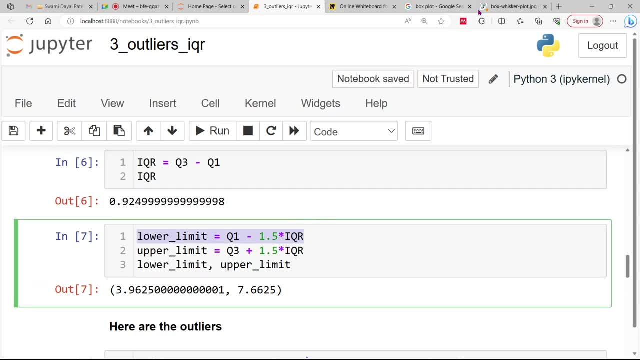 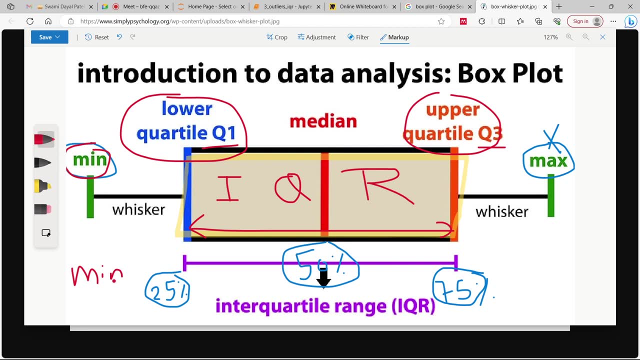 value, which is 0.95 lower value in this graph, it's giving minimum right. so minimum is what? minimum is not the minimum value. let me explain again. it's the Q1 lower quartile minus 1.5 multiplied by IQR. the formula is fixed for every data set. as far as maximum value is concerned, it's again not. 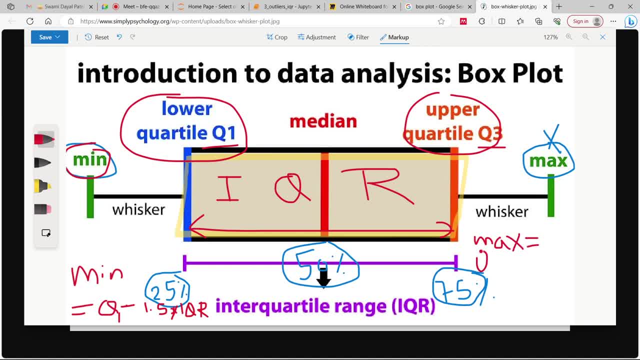 the maximum value of given data set, but it's Q3 which is on the right-hand side, plus 1.5 times IQR. you can write it down, this formula: we have just calculated what we have first calculated. go again. first we have calculated Q1, which is the first value. then we calculated Q3. 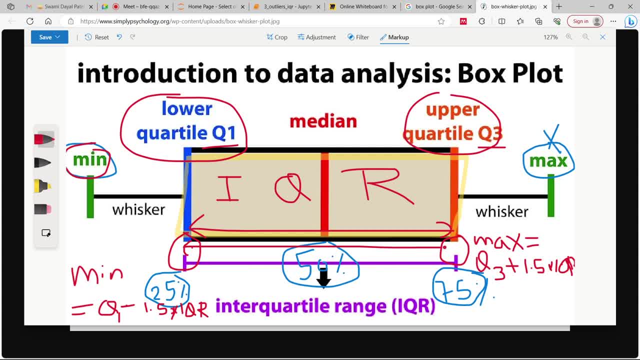 which is 7.5 percentile. then we find the difference between these two. what's this value? this is IQR for us. then we subtract this q1, which is this point, from this q1, we just subtracted 1.5 times of IQR. for this q3, we added 1.5 times IQR. 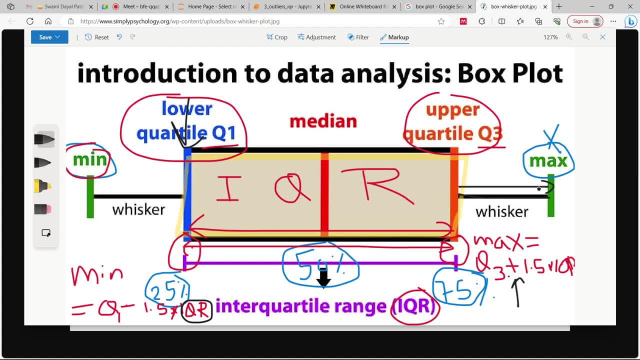 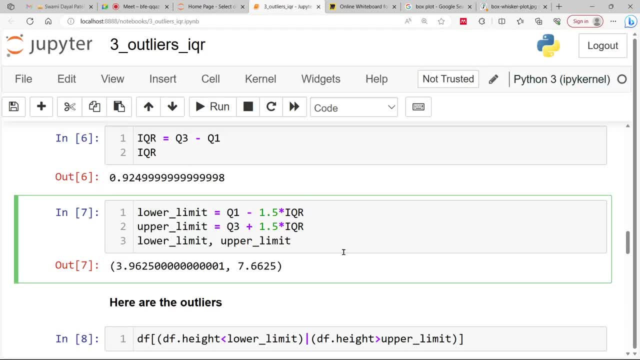 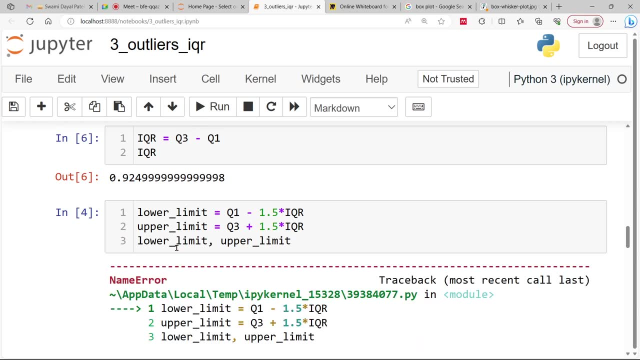 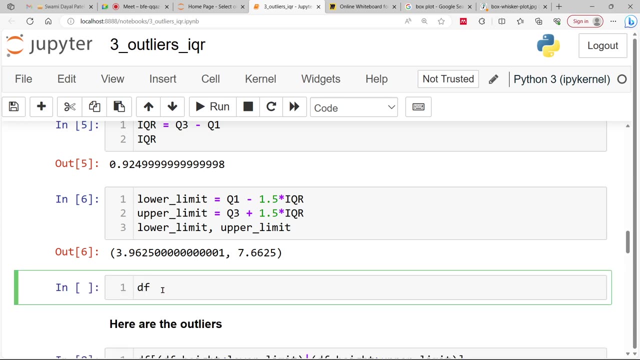 which is beyond this value. whatever value you are getting, that is minimum and maximum value. it's not the minimum and maximum directly. can you? can you analyze this when you? this is 3.96, something, right? okay, let me first, but if you'll check the df, and then we have codes h, e, i, g, s, t. 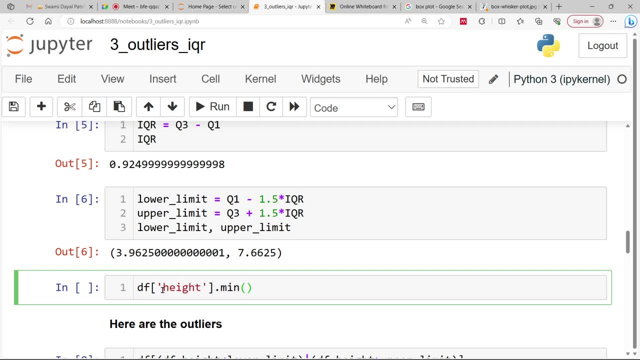 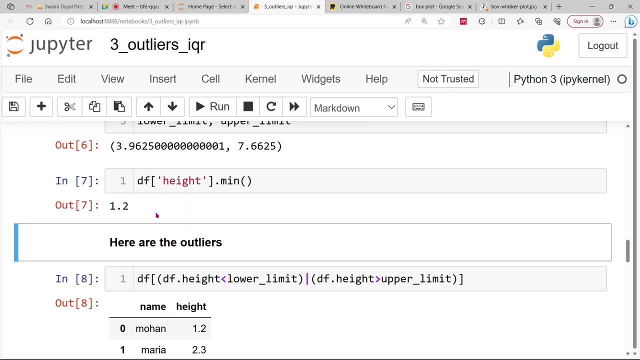 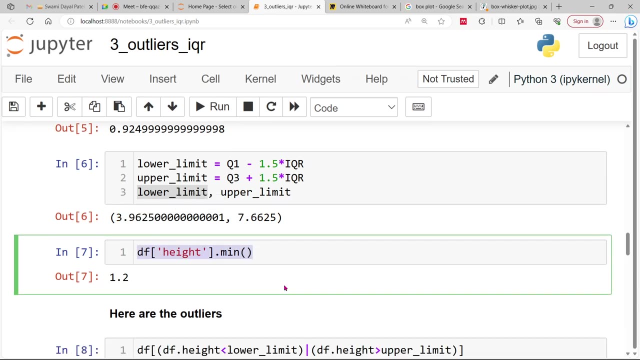 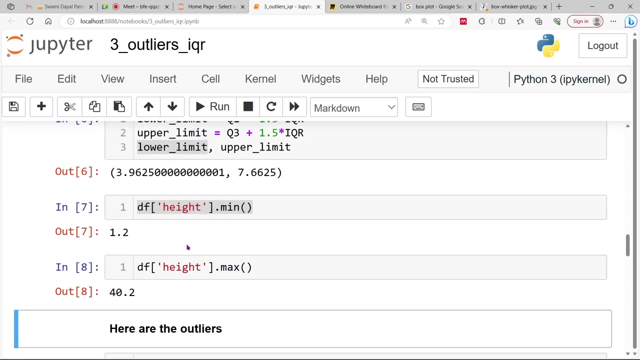 and this is minimum value. correct value: yes, df, and let's hide when you will check the minimum value, it's a 1.2, but we have lower limit as 3.926, which is not equal to each other because it's a conceptually different value. if you will check the maximum value, here max. so here we have maximum 40.2. 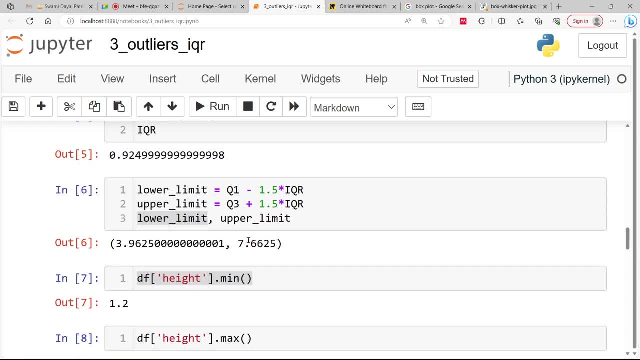 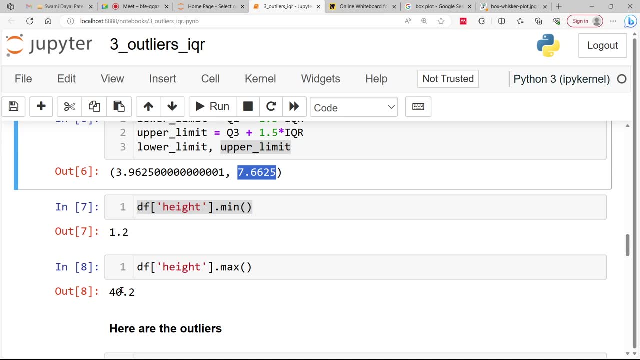 in the given data set. that's the maximum value, but we are getting upper limit as 7.2, 7.6, which is far away from this. 40.6, 40, 40.8. right now we are going to find out the outlets. 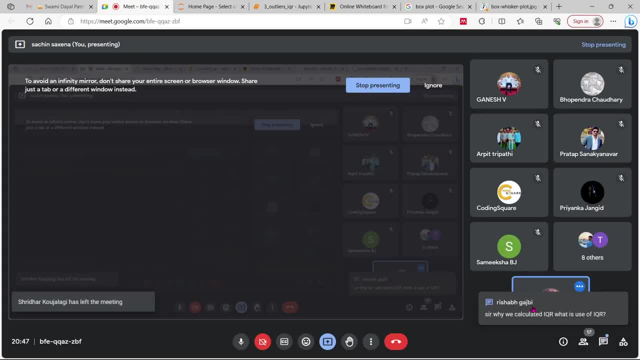 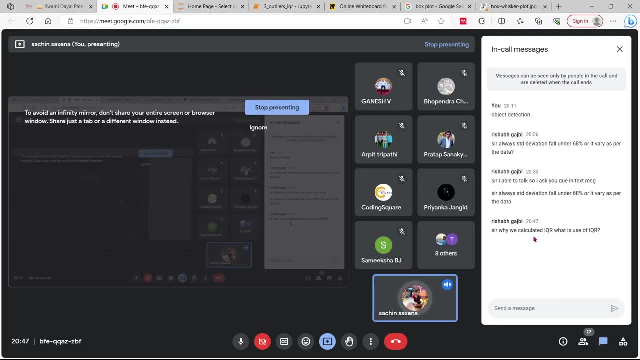 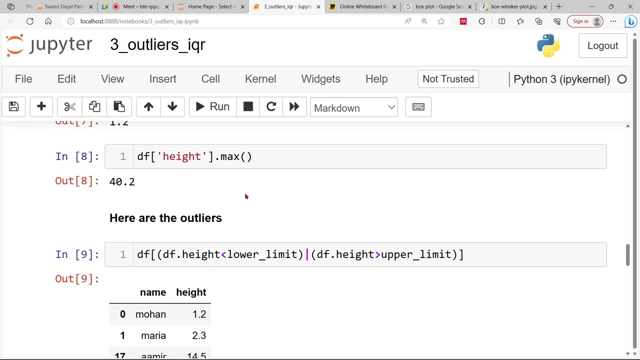 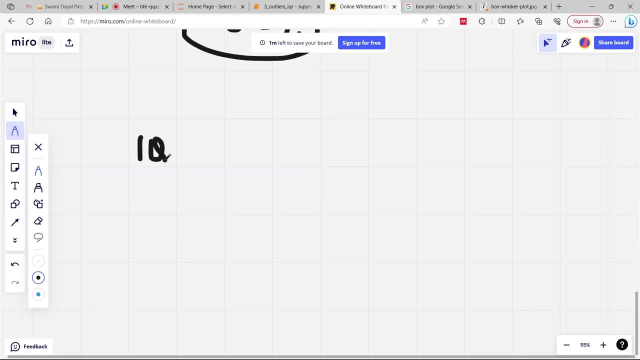 which is the point. yes, yes, rishabh, okay, sir, why we calculate IQR? what is IQR? okay, IQR simply the difference between 75 percentile. okay, it suggests just simply: IQR is just simply 75 percentile, like 75 percentile minus 25 percent. it's a fixed formula, right? yeah, formula, fix a he box, plot it, this, this, this plot. 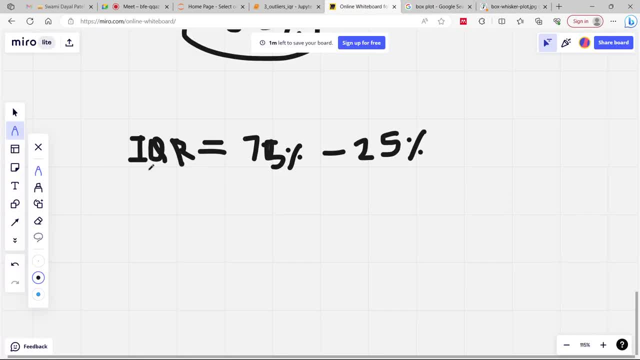 is called box plot here kills you. so when, whenever any interviewer will ask what is the formula for yqr, you will say: we calculate. first we calculate q1, which is this one 25 percentile, then we calculate q3, which is 75 percentile of whole data set. then we find the difference between these two and we call it this: 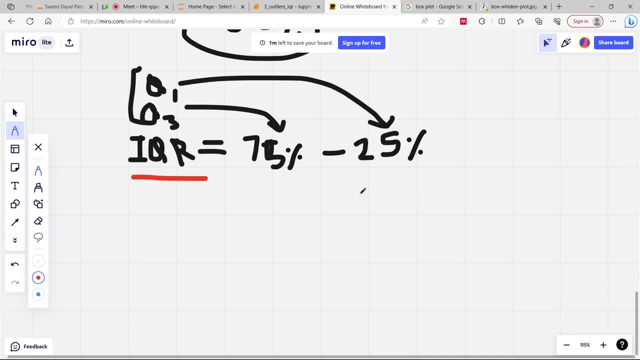 difference as IQR. this is the simple, simple step. then you will have to find the minimum and maximum value. so you will say, sir, this minimum or maximum value is not its respective minimum or maximum. rather, minimum is what? q1 minus 1.5 times iqr, whereas the formula for maximum is q3 plus 1.5 times iqr. did you get this formula? this is just summarizing of box plot. apart from this in box plot, any formula will be used in box plot. 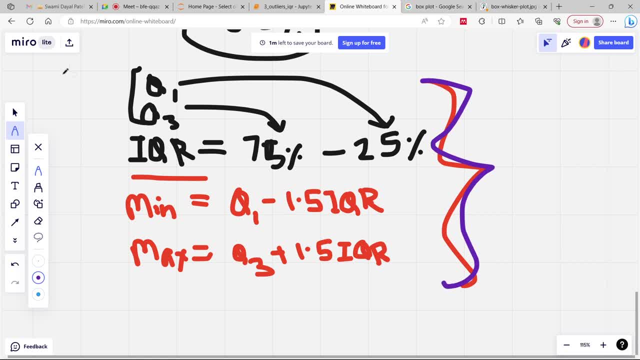 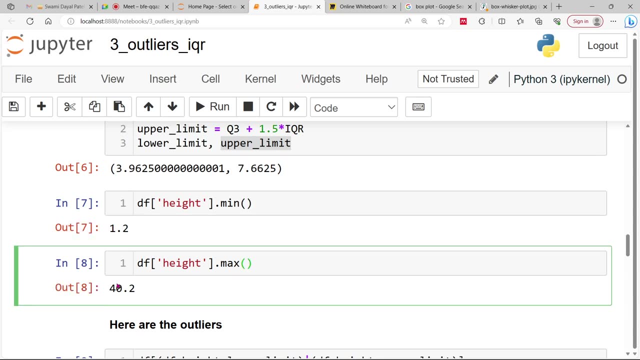 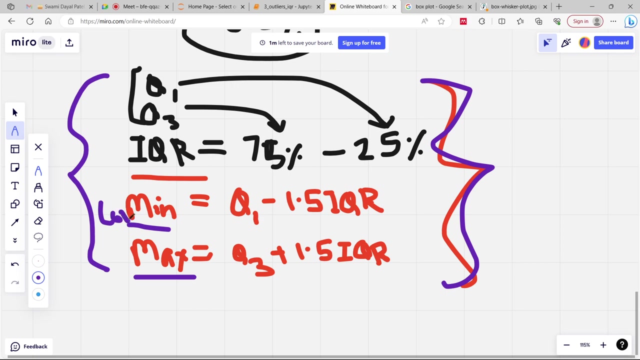 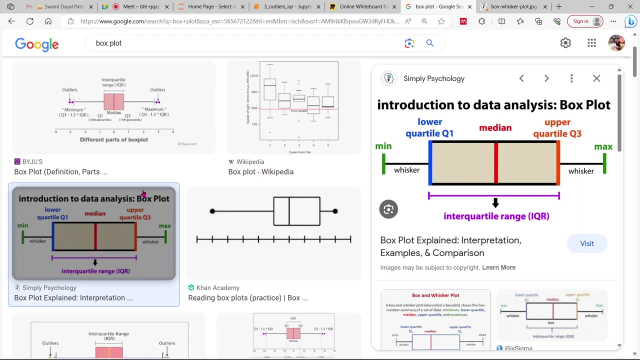 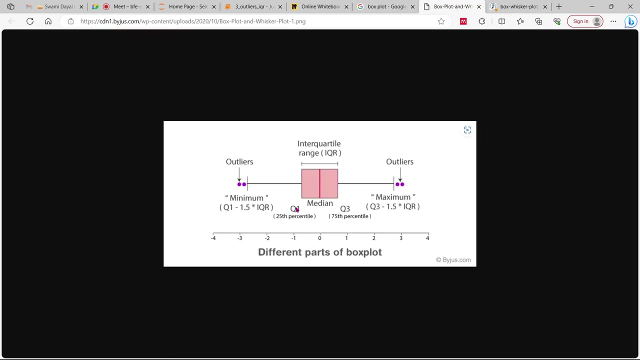 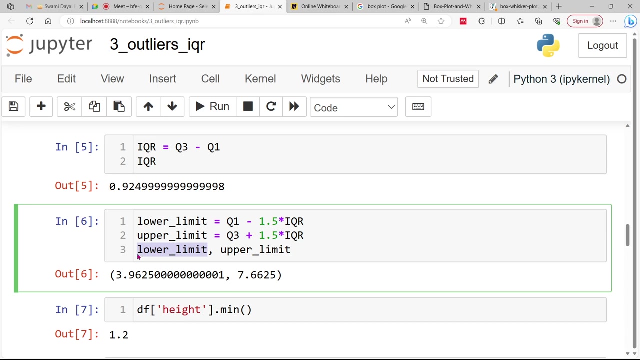 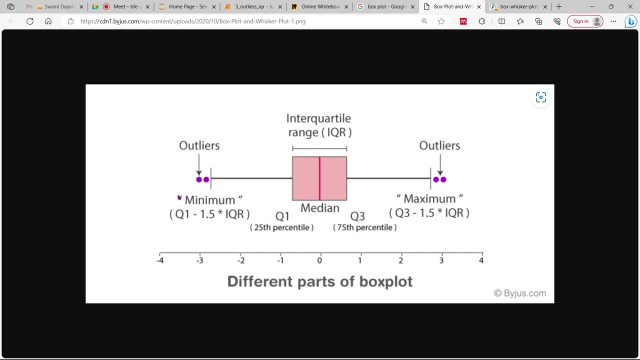 is it upper limit, this one right, which means in this box plot. you can see here also this. in this image you can see outliers jo in minimum and maximum, ke beyond values. hoti hai, like jo value, which value is beyond this lower and upper limit? 3.96 and 7.66. that is called outlier for you and you want to. 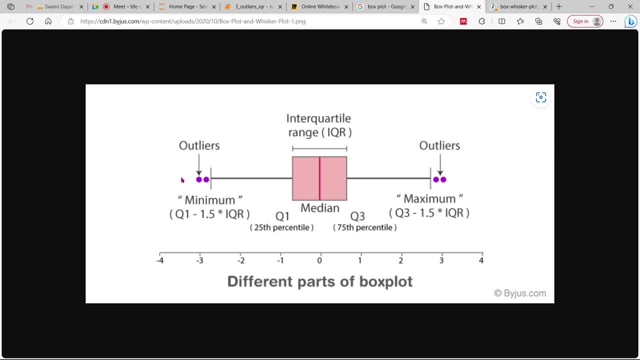 remove this outlier, so iss outlier mein minimum bhi include hoga. aur right hand side outlier mein maximum bhi include hoga, which is the only which is justified my earlier statement which it's not the same minimum and maximum. hence you are going to remove all these values. 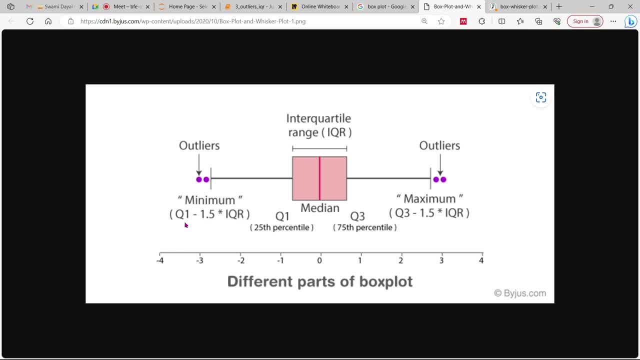 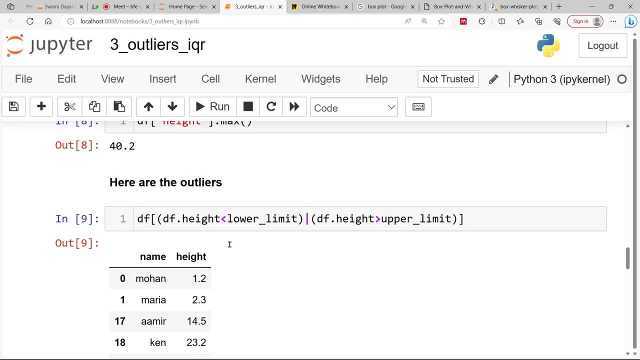 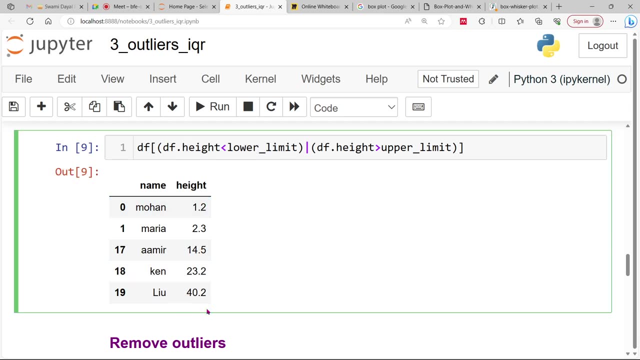 minimum and maximum, which is beyond first data and second, minimum, lower limit and upper limit. alright, now go back here. here we have all these terms: jo ye, candidates, hai. they are not following this lower limit and upper limit, so we need to remove the these five candidates. enko, bahar, nikaalo. then you have clean data set without outlier. now.